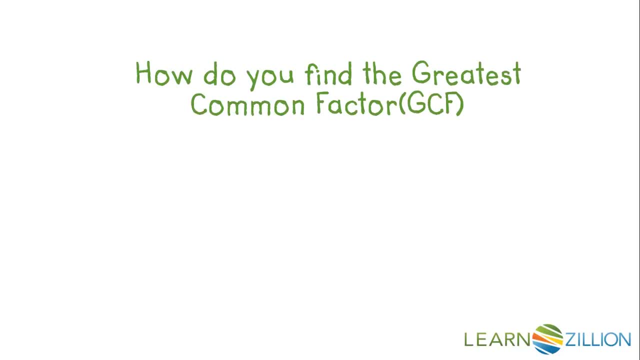 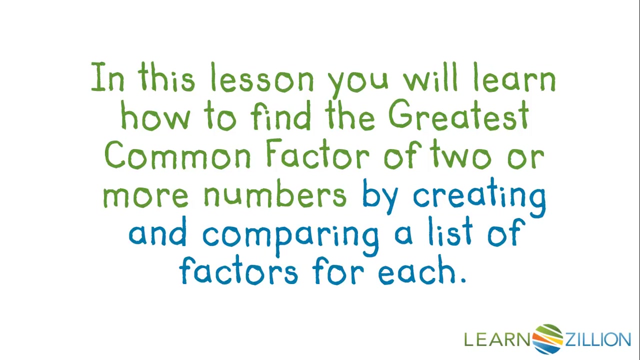 How do you find the greatest common factor, or GCF, of two or more numbers? For example, how do you find the greatest common factor of 32 and 60?? In this lesson, you will learn how to find the greatest common factor of two or more numbers by creating and comparing. 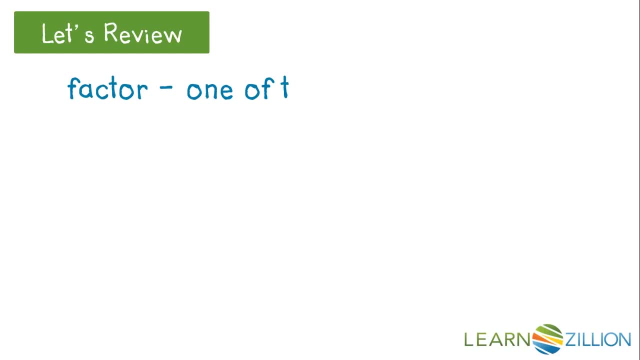 a list of factors for each. Remember, a factor is one of two whole numbers that, when multiplied together, result in a product. If I want to find the product of 15, I can list the facts of 15, the multiplication facts, and then I want to make sure that I create a list. 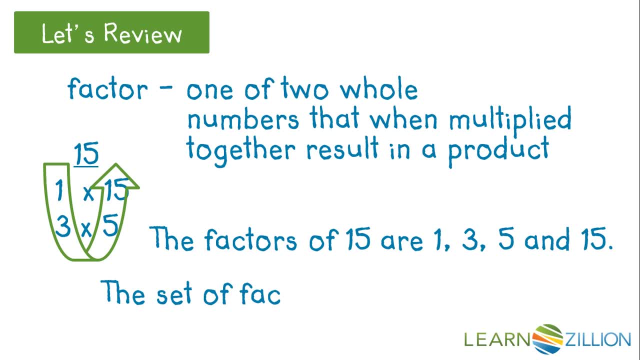 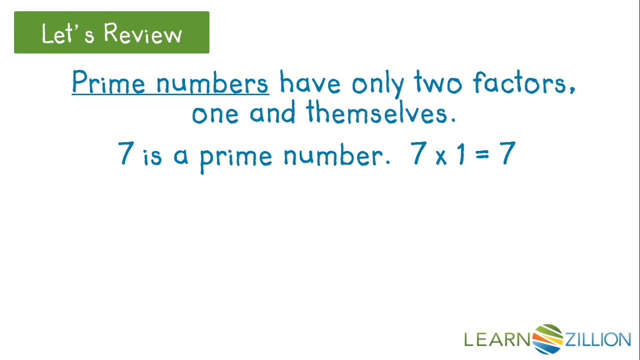 of the factors themselves. I can even write this list as the set of factors for 15 by using brackets around 1,, 3,, 5, and 15.. Remember, prime numbers have only two factors. one is one and themselves 7 is a prime number, because 7 times 1 are the only whole number factors. 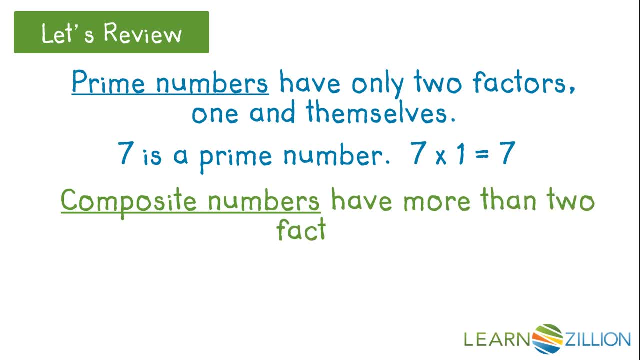 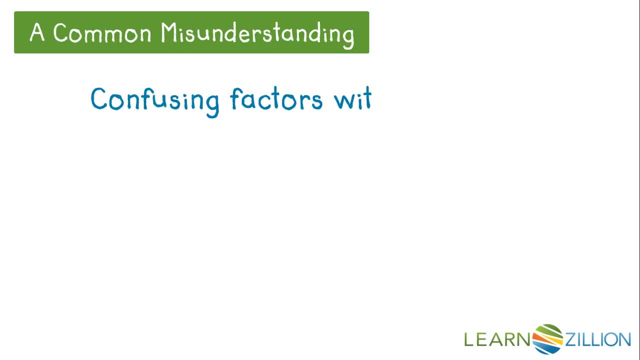 for 7.. Composite numbers have more than two factors. 10 is a composite number because it has four factors. A common misunderstanding when working with factors is to confuse them with multiples. If I was to ask to find the factors of 25, which list would be appropriate? 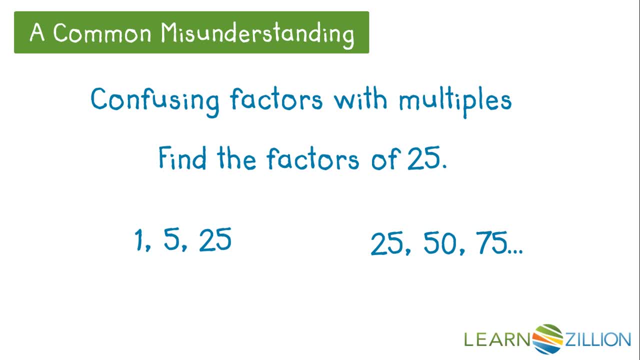 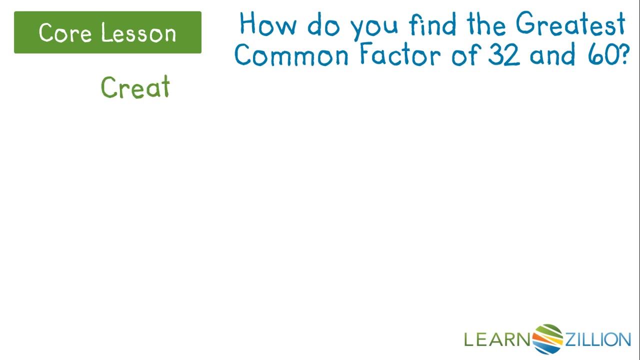 Of course, we're looking for the pairs of numbers that, when multiplied together, give us the product of 25.. So I would not want to use the skip counting multiples. Our original question was: how do you find the greatest common factor of 32 and 60?? Well, 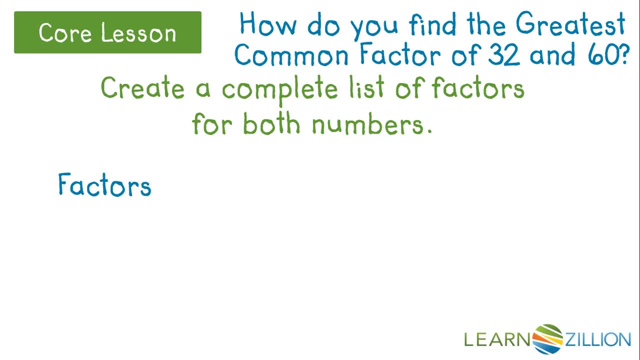 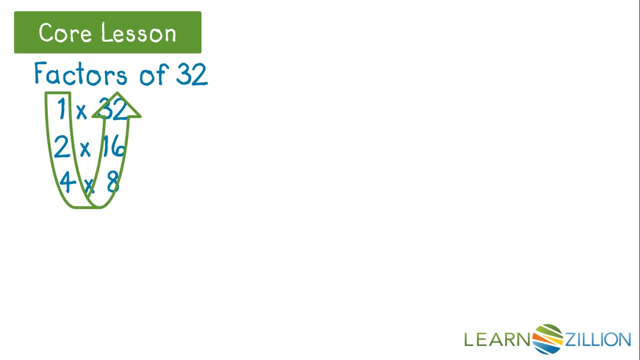 I'm going to create a complete list of factors for both numbers. Alright, I have the facts for 32 here and the facts for 60 coming up on your screen right here. So now, when I look at the facts of 32, I want to list them in order from smallest to largest, So I know. 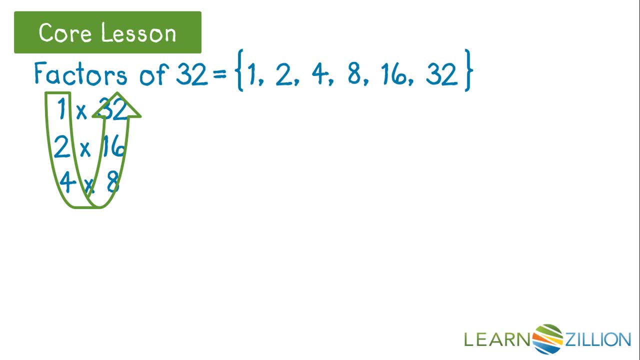 that the set of factors of 32 is 1,, 2,, 4,, 8,, 16, and 32. inside brackets I know that the facts of 60 are listed here. I want to follow those facts around to range them in.